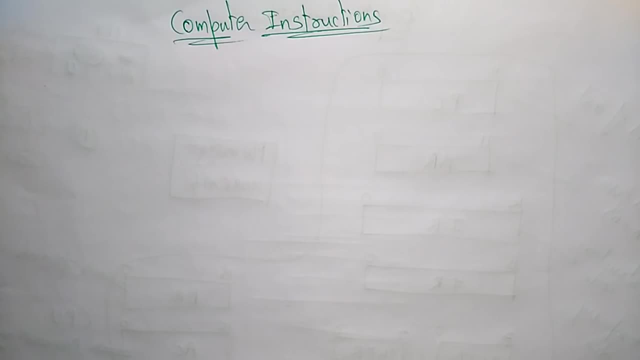 Hi students, let us continue with the topics of computer organization and architecture. So coming to the next topic, that is, the computer instructions. So in the previous video I explained about the computer registers, different registers that are present in the system computer. Now let us see what are the computer instructions that are present in system. 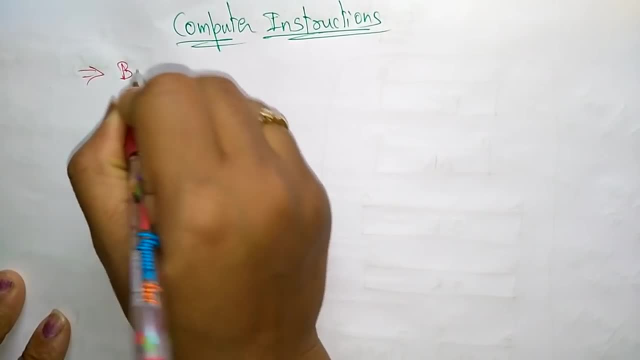 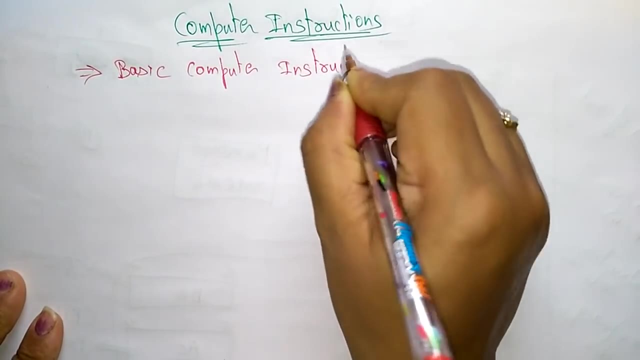 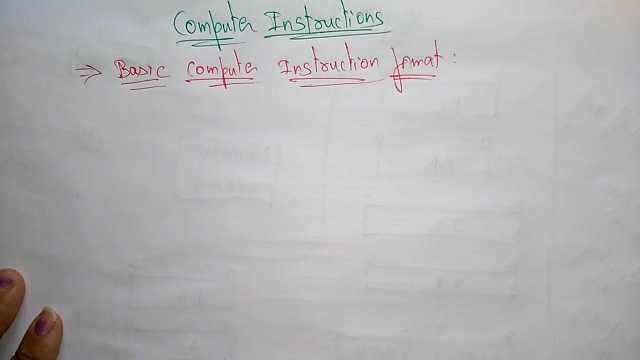 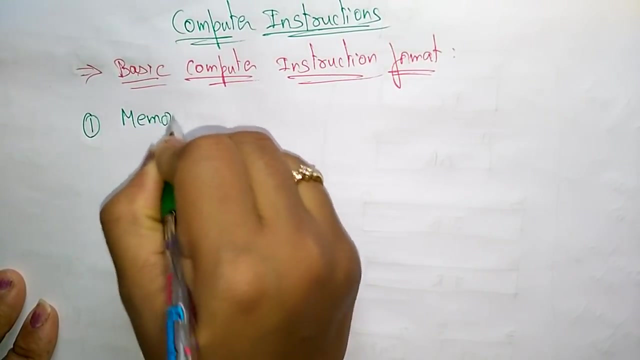 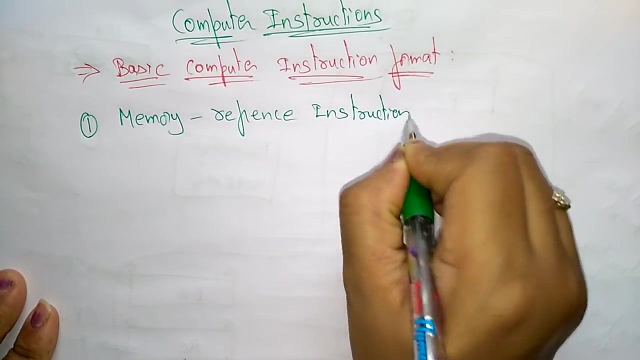 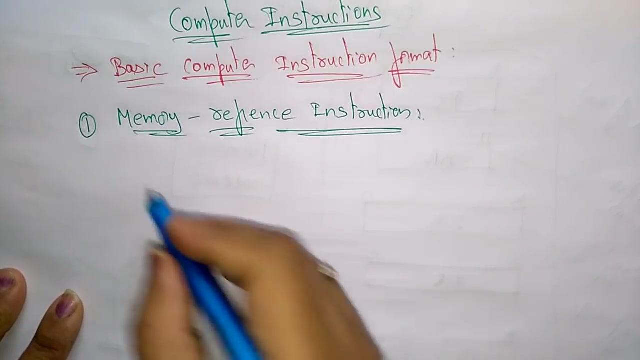 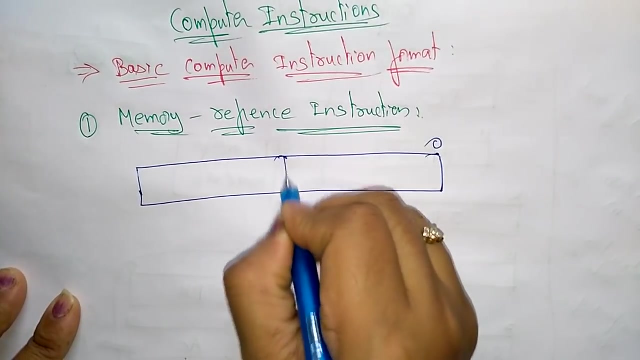 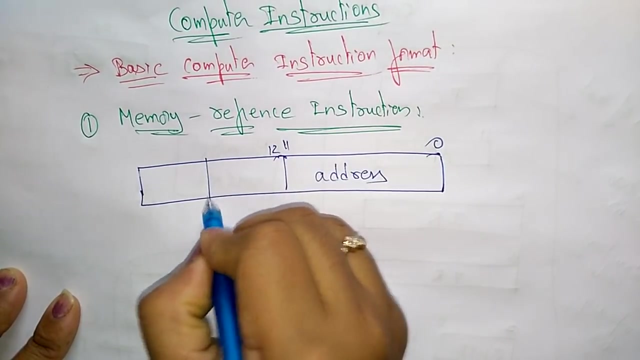 So the basic computer instruction format is basic computer instruction format is three types. There are three different formats will be used in the computer. So one is the memory reference instruction. So the first format is the memory instructor reference instruction. So this memory reference instruction will be. so. this is a 16 bit register. It holds the data. from 0 to 11 occupies the address of the memory to where the data has to be stored, and 12 to 14 bits means these three bits indicates the op code. 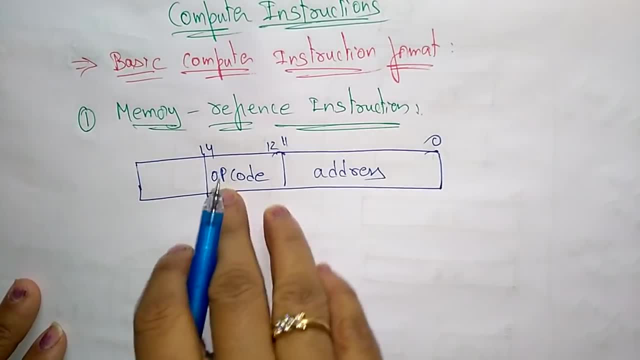 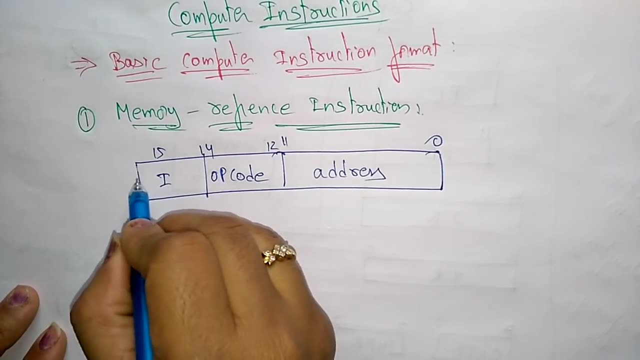 Op code means what operation is there. it has to be performed. that will be indicated in these three bits. okay, and the last bit is the 15th bit is the i bit. so here, this i is nothing, but it is an addressing mode. it indicates the. 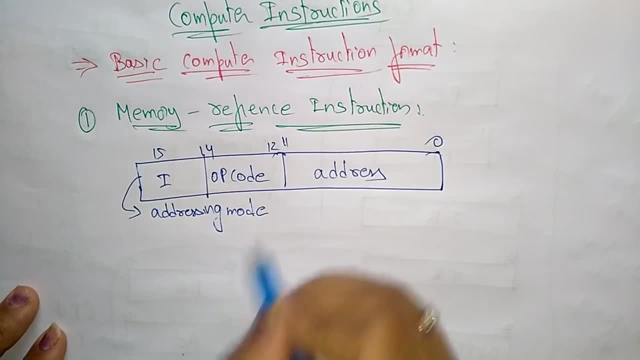 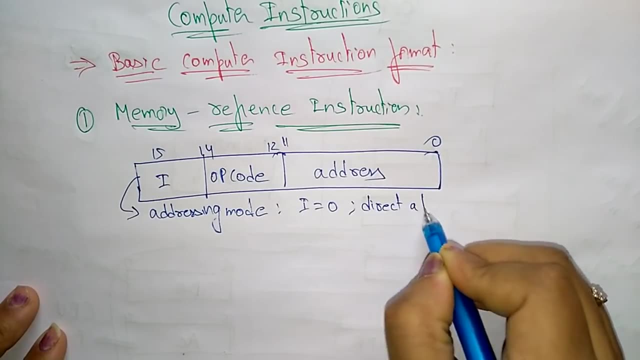 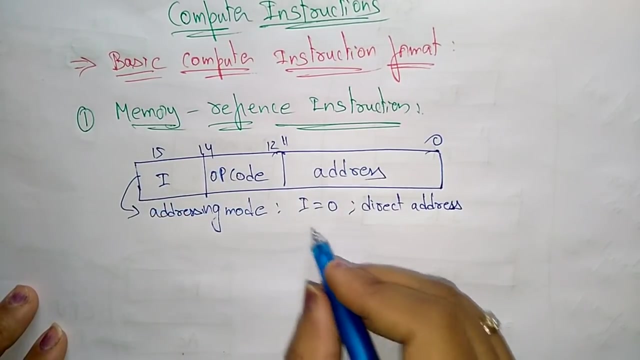 addressing mode. addressing mode, suppose if i is zero it's saying that it is a direct addressing mode. direct address means the direct address to where it has to be get. that will be stored in this. it indicates i is one means means whatever the address we are stored here is a direct address. 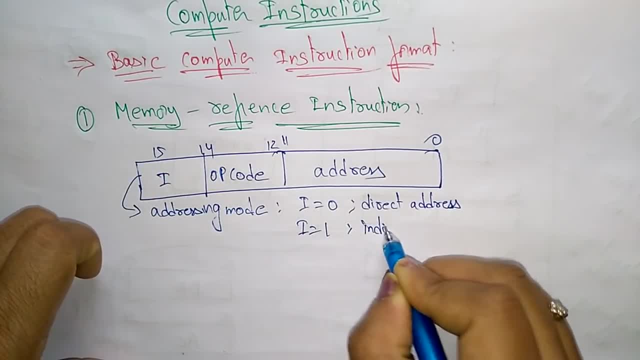 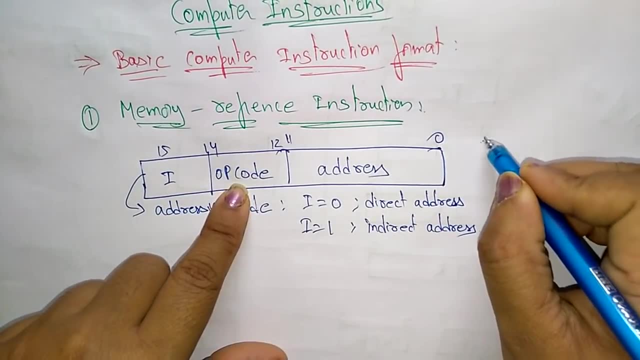 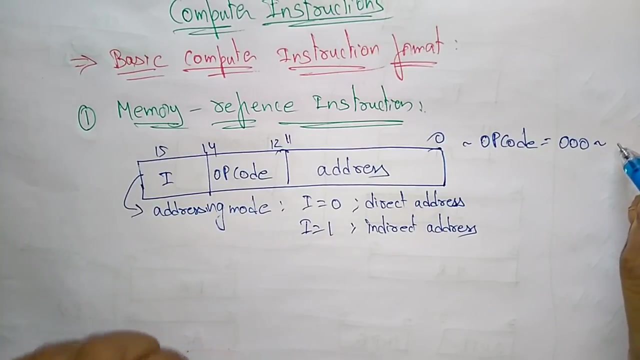 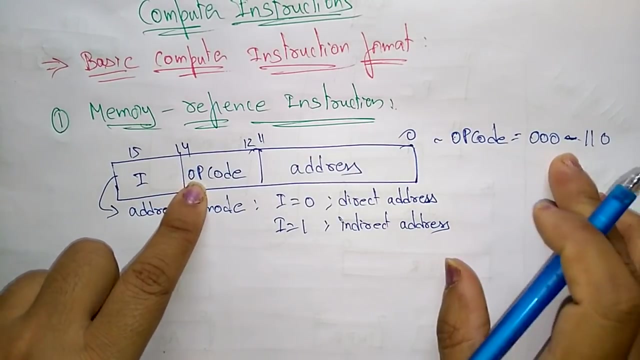 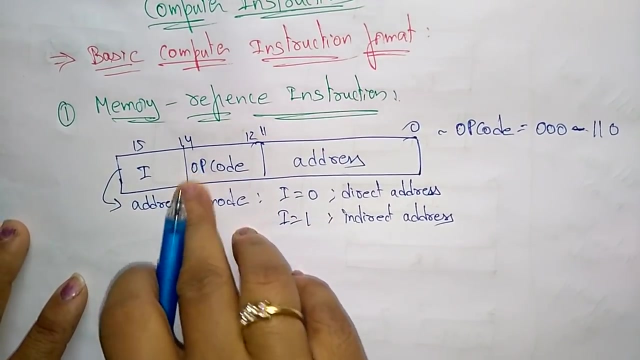 suppose, if i is one, it indicates it is an indirect address. okay, so here the opcode. this opcode should be is in the range of: from 0002. it store up to 110, 0 means up to 6, 6, 6 bits, so 0002, 110. these complete opcodes will be stored in 12 to 14 memory. reference instruction. 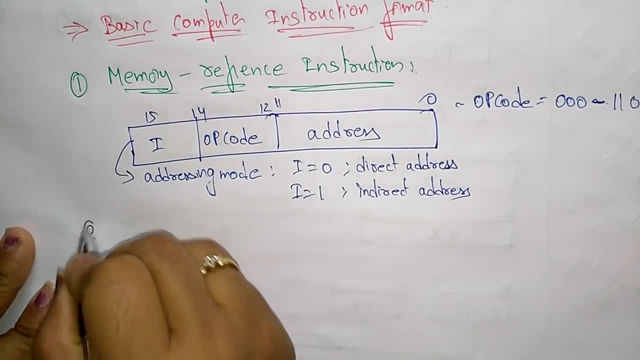 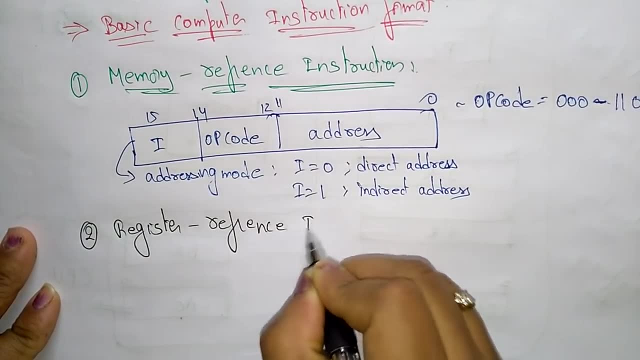 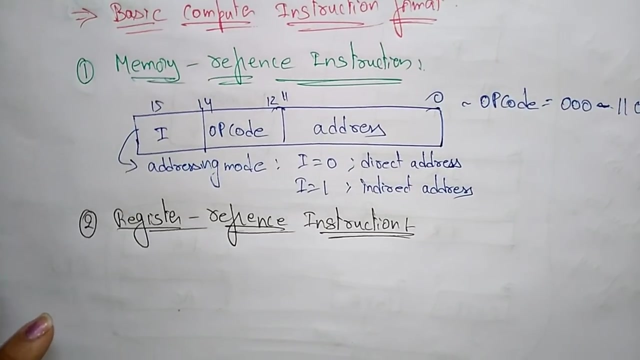 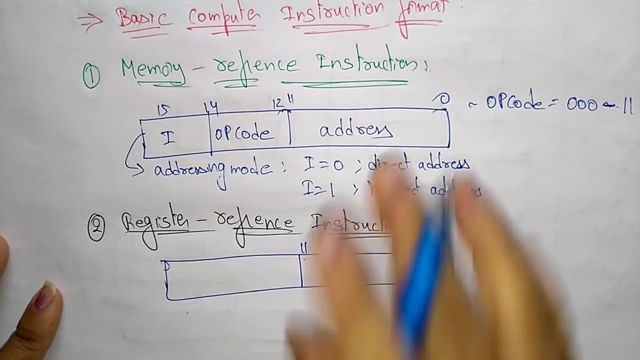 now coming to the next instruction- this is the second. one- is a register reference instruction. register reference instruction. so let's see the format of register reference instruction. so this is also sixteen bit. so zero to eleven here in memory reference instruction. the zero to eleven occupies the address. 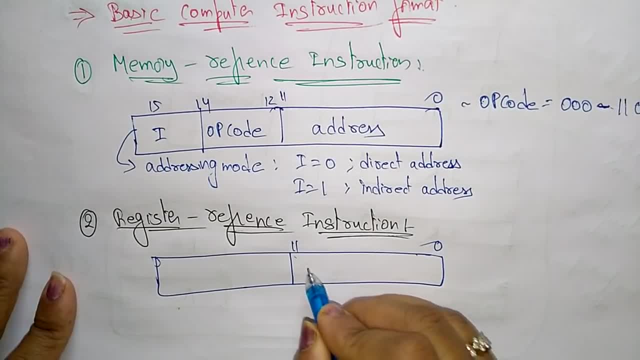 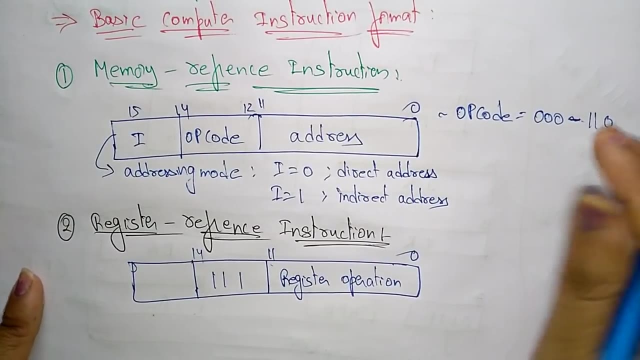 whereas register reference instruction. the zero to eleven occupies the register operation what operation the register has to be performed that will be stored in zero to 11 and twelve to fourteen indicates the one one, one means zero, zero, two, one one, zero. it occupies the memory reference instructions, whereas the last one, one one ubis, which is in the register operation operation. 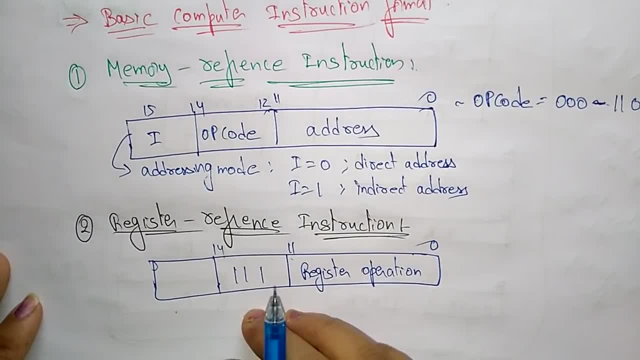 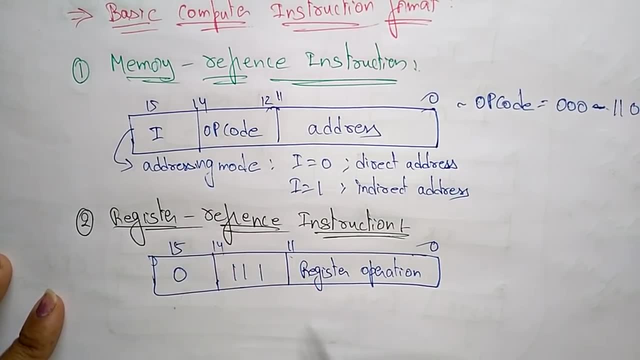 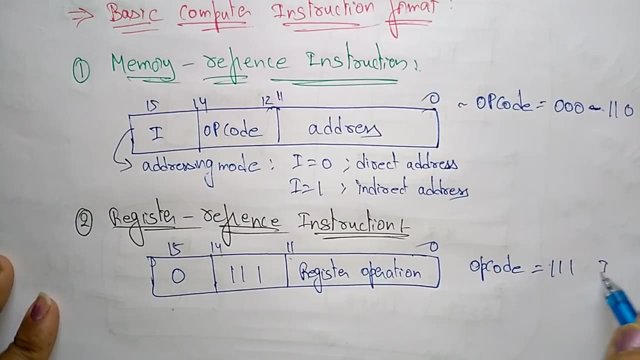 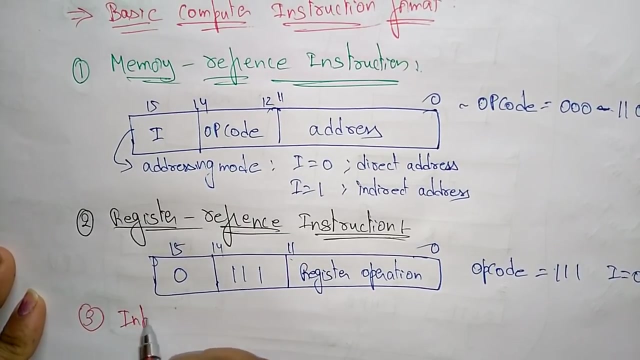 whereas the last 111 will occupies the register reference or I-O reference, and for register reference always the 15 bit should be 0. So here the opcode is 111 and the I should be 0 in register reference. Now coming to the next one is input output reference. input output. 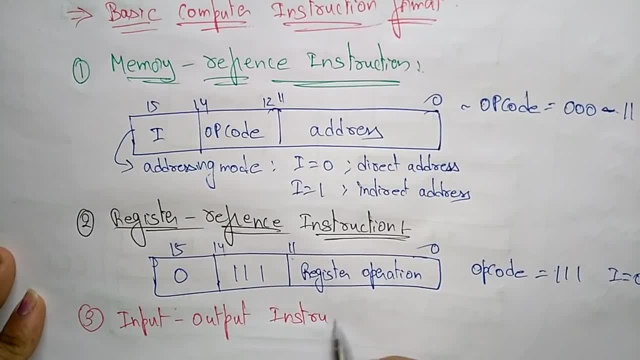 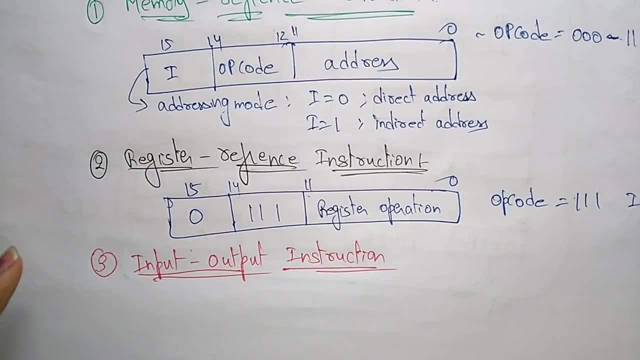 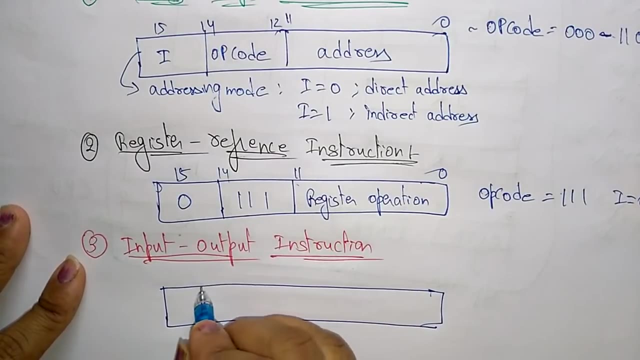 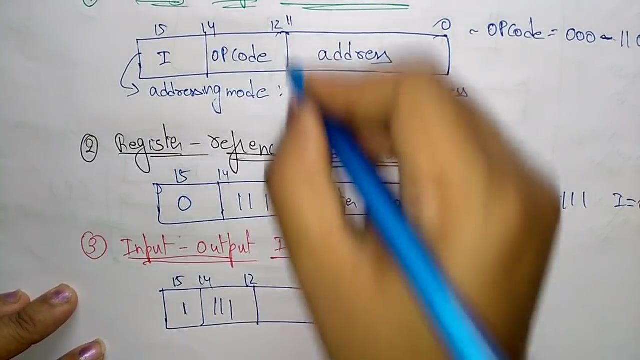 instruction. So what is the format of this input output? the same as the register reference, but instead of 0, the I bit indicates the 1, and 14 to 12 it occupies 111.. So this is the same, but only the difference is the 15th bit. if it is 0.. 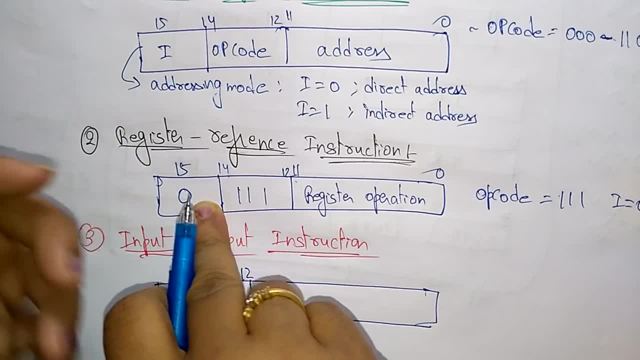 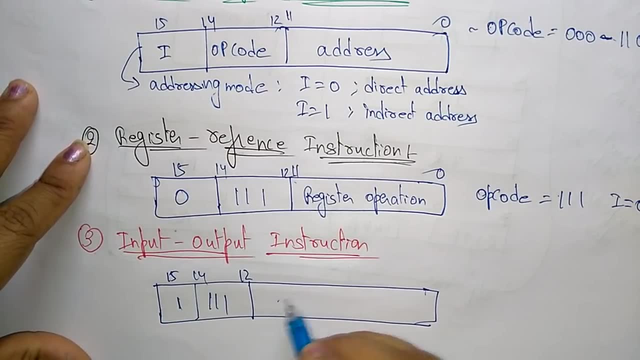 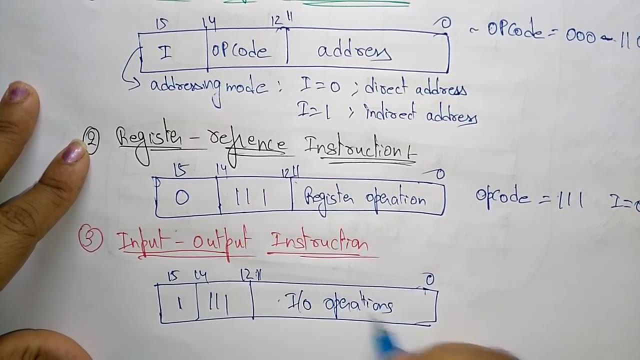 you have to perform register reference instructions, you have to take the data as register reference instruction, whereas it once indicates it is an input output instruction and here, from 11 to 0, it holds the IO operations. so here also, the opcode is 1, 1, 1 and I should be 1. so this is the 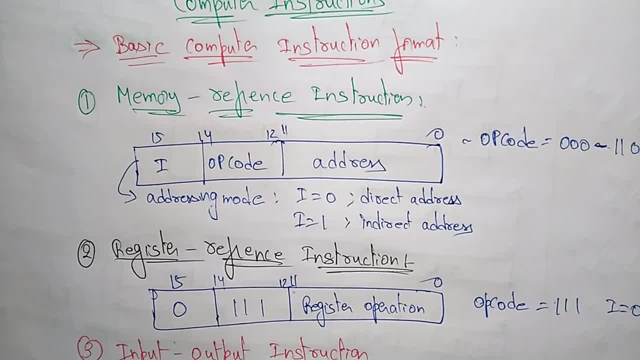 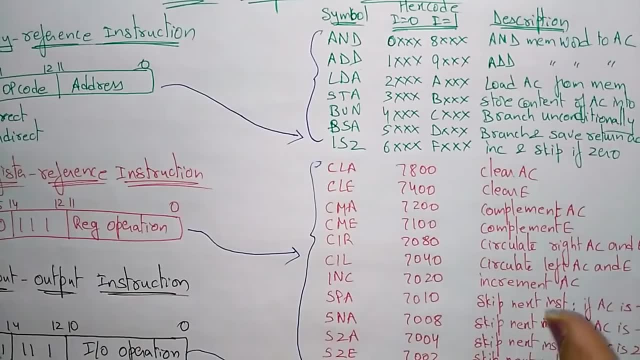 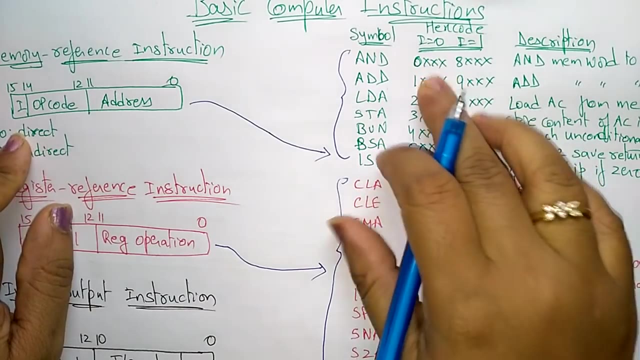 basic computer instruction formats. now let us see some basic computer instructions format. what are the instructions that are stored here? so here i is equal. 0 or 1 indicates whether the it is a direct or indirect addressing. it holds the exa code okay. from 0 to 6 it indicates a. 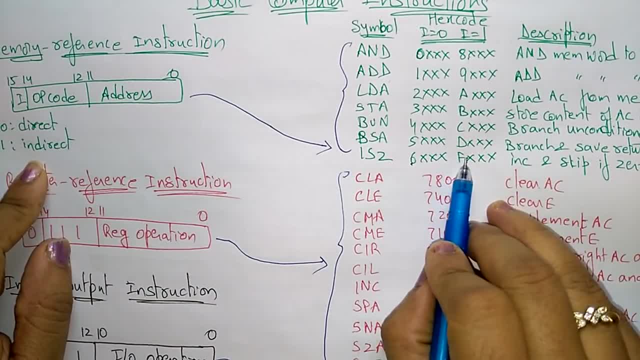 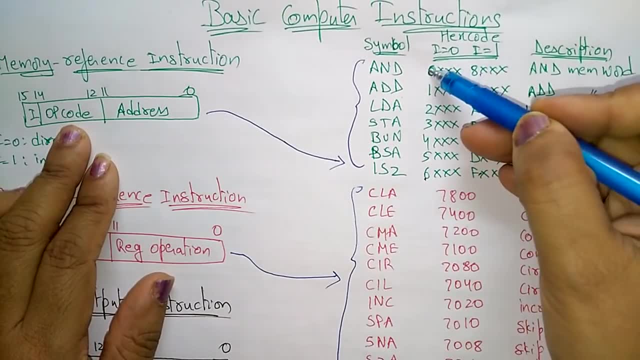 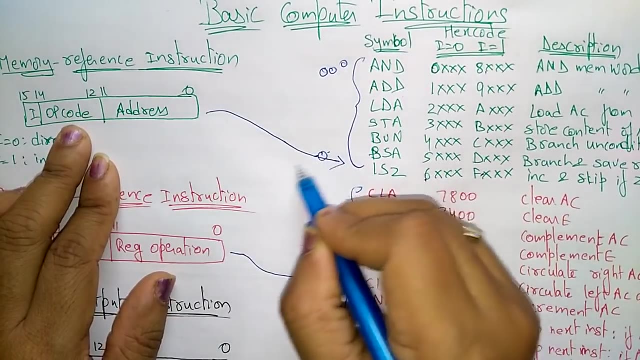 direct addressing, whereas 8 to 15 it indicates the indirect addressing. so the memory references translate will hold. the opcode is from 0: 0 0. 0. 0 to 6 means 0. sorry, 1 1 0, 1 1 0. so here this is, I am saying: 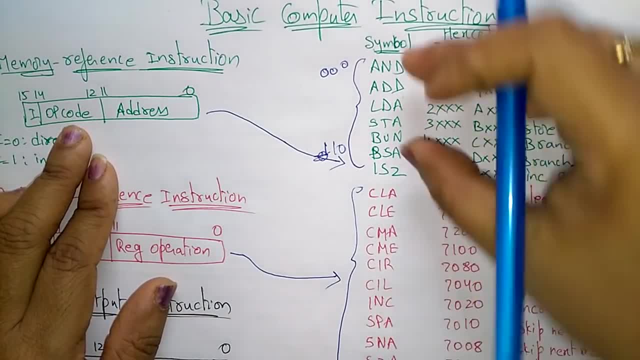 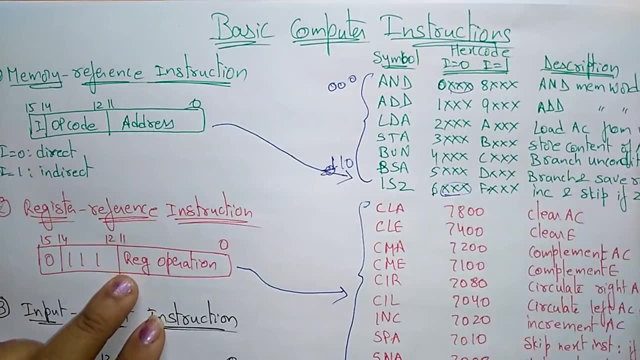 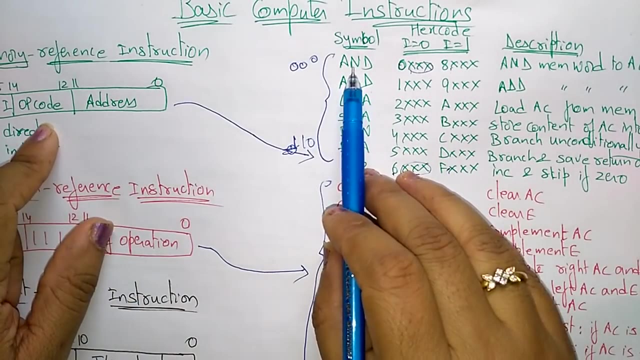 about this: from 0 0 0 to 1 1 0 will holds the opcodes these instructions will refer to as a memory reference instruction. so up to this, green color is indicated as a memory reference instructions. okay, so here the opcode end and indicate end memory word to accumulator. so 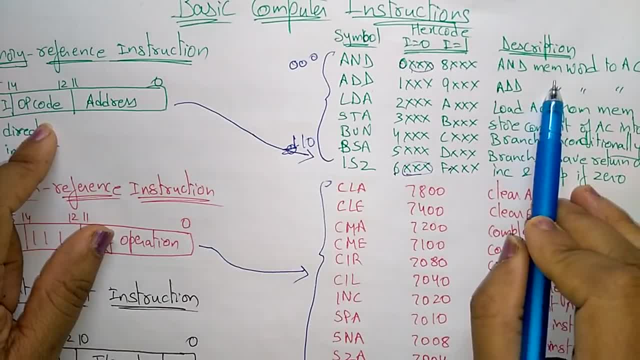 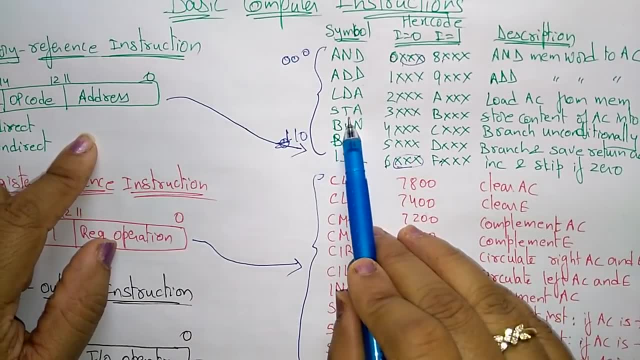 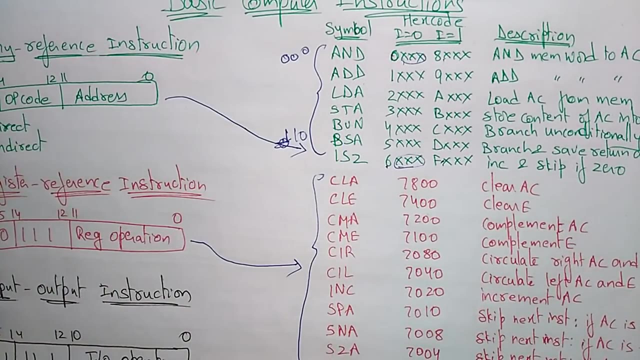 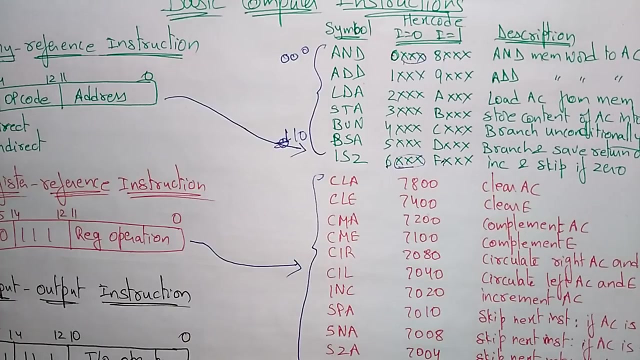 whatever the end word memory word should be there. that has to be ended with the accumulator add. LDA means load accumulator from memory, SDA means store content of accumulator into memory. so accumulator is a register which holds the result of an operation. so always the result will stored in the accumulator register in the processor, so which is present. 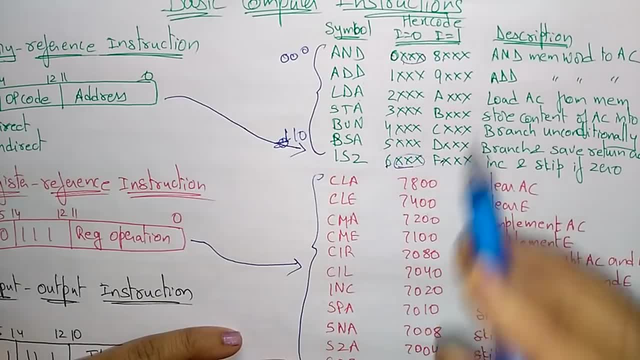 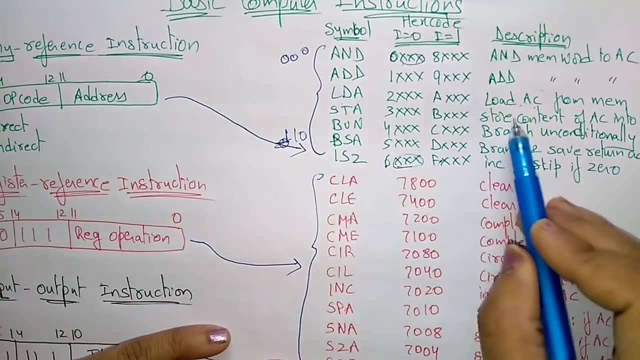 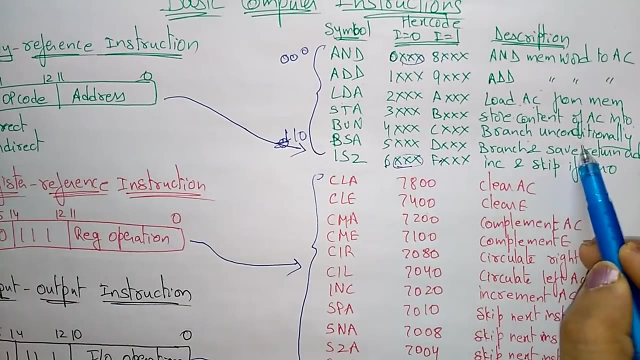 in the processor. processor construct of registers in that register accumulator is a, holds the result. so load accumulator from memory, store. store content of accumulator into memory means you are copying the data into memory. BUN means branch unconditional, BSA branch and save written address. ISJ is nothing but increment. 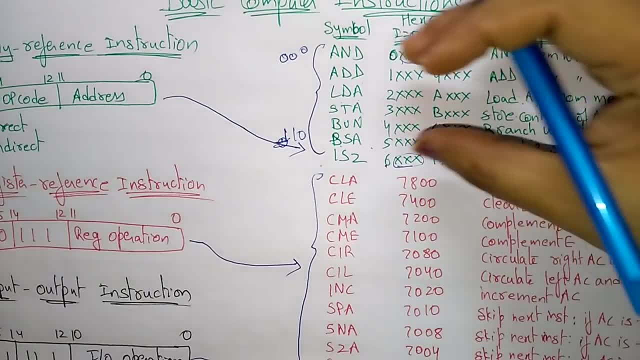 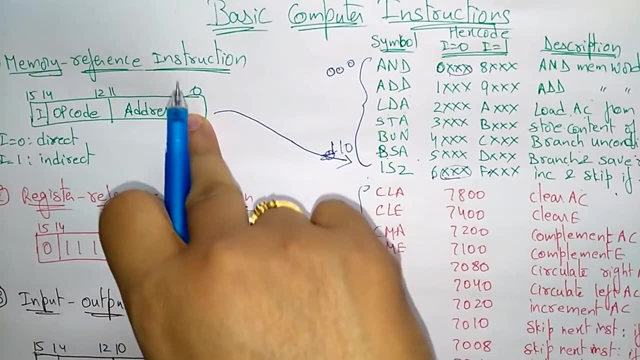 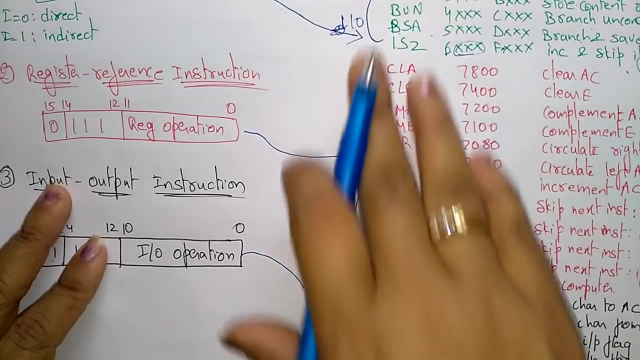 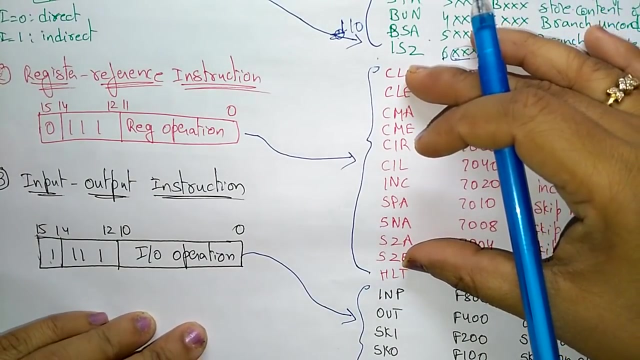 and skip. skip if 0. okay, so these are all the operations that are referred to the memory reference instructions. so these are the memory reference instructions. now coming to the register reference instruction, which instructions you call it as a register reference instruction? so all these complements and a circle, circulate and skip. these are all comes to the register difference instructions. 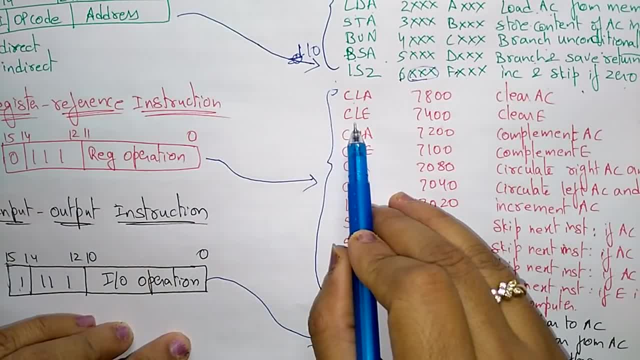 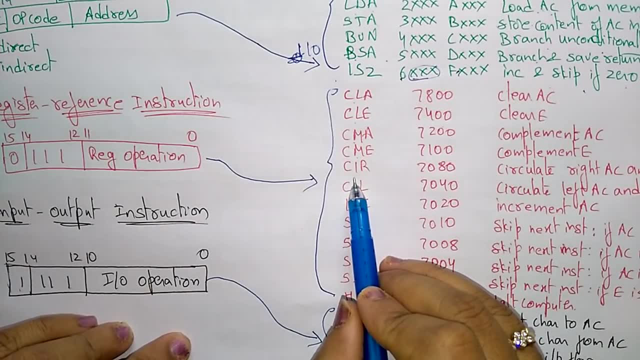 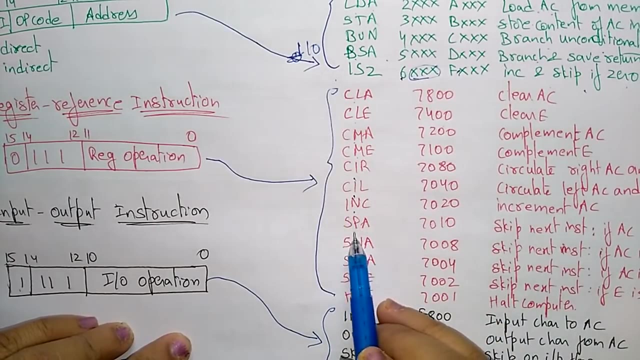 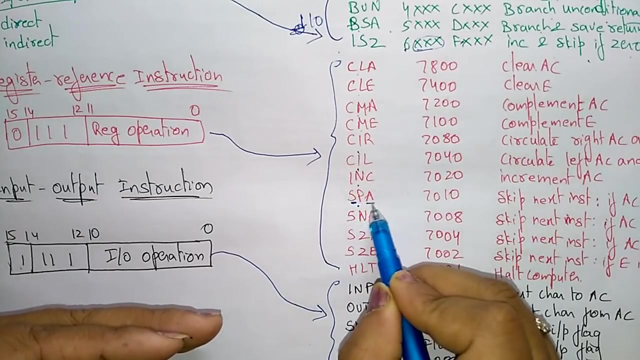 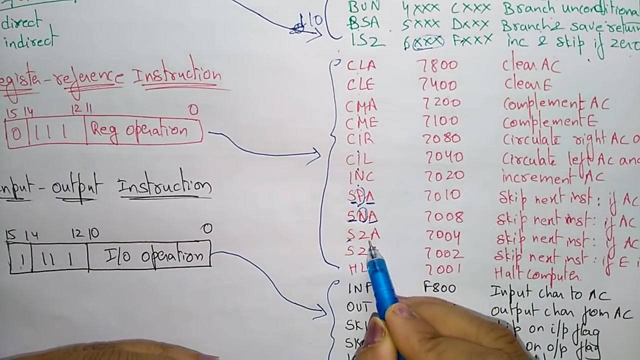 so this is clear accumulator, clear E compliment accumulator. compliment II: this is circulate write accumulator and e circulate left accumulator and e. this is increment accumulatoras. PA means it skip to next instruction. means: if accumulator is positive, skip. if accumulator is positive, skip if accumulator is negative, skip if accumulator is 0.